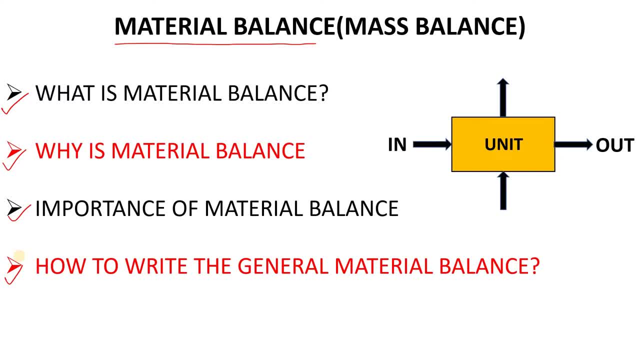 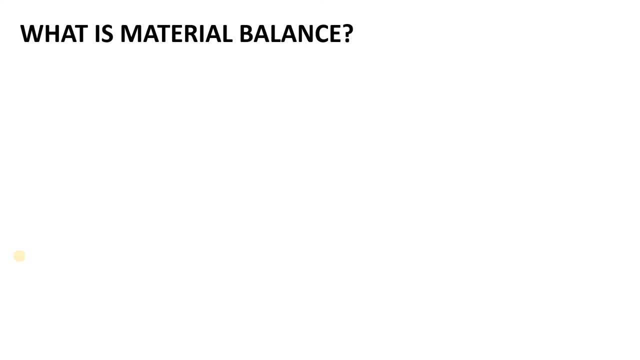 So let's start the video from what is material balance? So first we start from the definition of the material balance, right? So the definition of the material balance is here. You can see that material balance is an application of the conservation of mass means. it depends, or it. 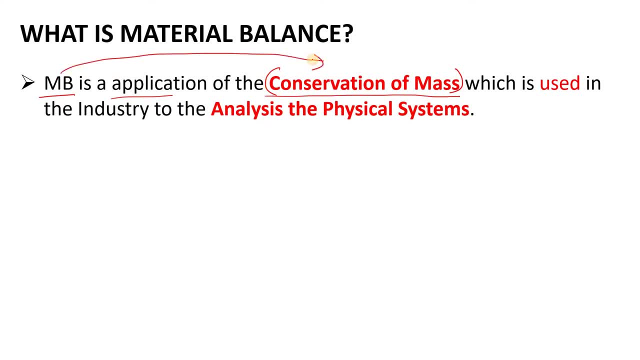 based on the conservation of mass. and the conservation of mass states that mass can neither be created Nor destroyed. Got it my point? Suppose there is a reaction that is A plus B and it goes to C plus D, Then whatever will be the composition and we can say the amount here. Suppose, if there is a amount, 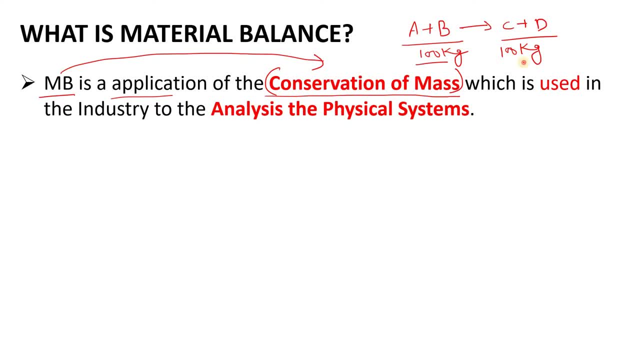 of these. both is 100 kg, So here will be also 100 kg. Got it my point Now ahead- which is used in the industry to analyze the physical systems. okay, So this is very, very important. So this is very, very important and we will see this via one example. It is used to analyze the physical 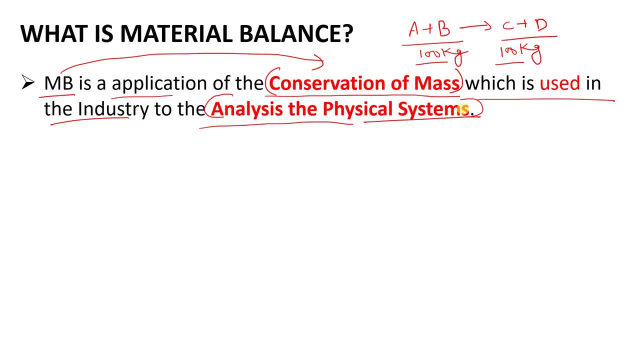 systems. What is this means? we will discuss this. we are one example, okay. So while you are solving the problems on the basis of material balance, So you should know that actually what you are doing, and if you are in the plant, so you should know that why we are using that. material balance. okay, If you know the why behind the whatever you are doing, So it is very well. It will be very useful. I'm going to talk about this material balance, Okay. so now we are going to talk about this material balance. 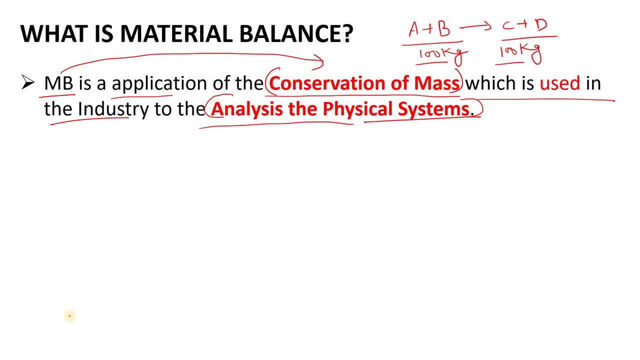 Right, So we are going to talk about this material balance. So let me give you a basic idea. the material balance is going to be that of these two types, One is not a steady material balance. okay, the whatever you are doing, so it is very well. it will be very, very important for you to do that. 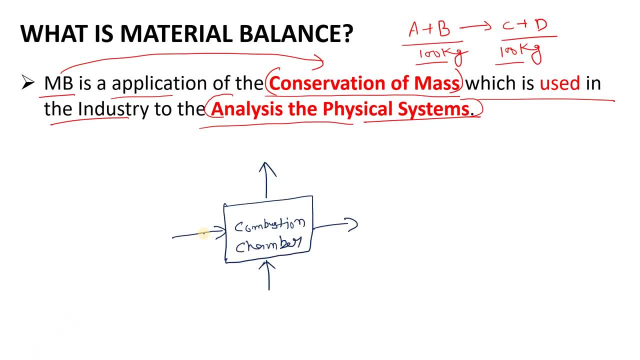 work okay and it will be joyful for you. let's see, here, this is my combustion chamber. okay, there is my combustion chamber and here i supply some feed. okay means you can simply say wood, okay, i am supplying the wood. so wood consists of carbon, and we can say simply s: okay, and here i'll get the 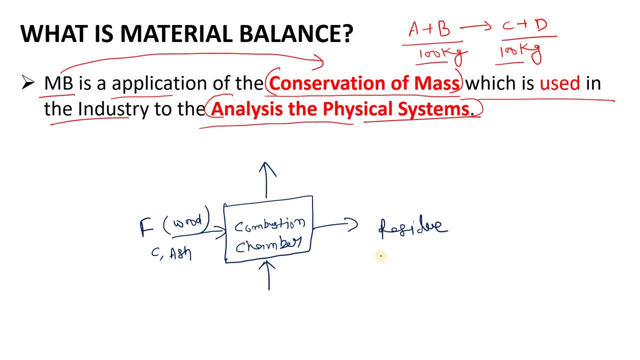 residue. okay, and in the residue there will be mainly s got it my point. and there will be some amount of carbon as well. so it will be in a minor amount. and what we supply here, we supply the air and what we get, we get the flue gases or we can say the stack. 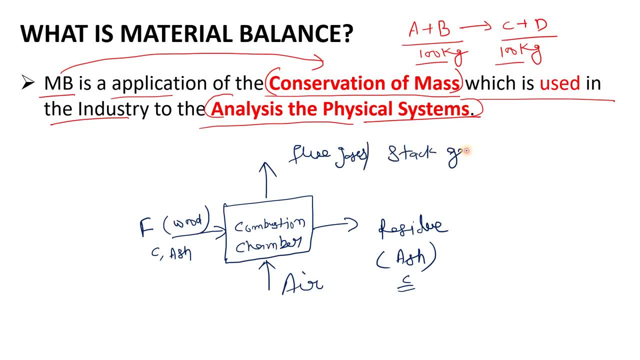 gases got it my point. so, with the help of this material balance, we can find out the quantity, quantity, quantity. we can find out the composition- okay- of the residue here or in the residue. we can, i can find out the- what is the amount of s which is going to generate after the complete combustion? okay, 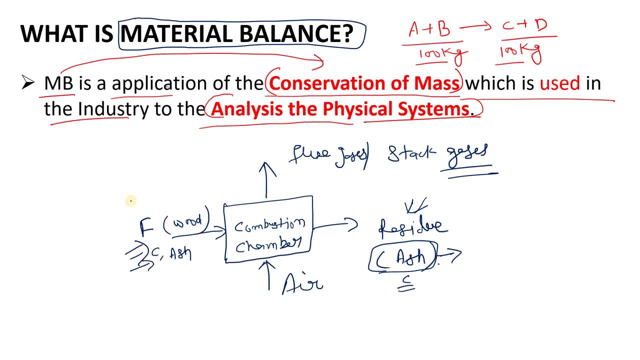 we can also find out the carbon quantity here if we know the feed. suppose, let, the feed is 100 kg. okay, so this is the beauty of the material balance. just i am giving one example and in our upcoming videos we will discuss about the physical systems. it may be. 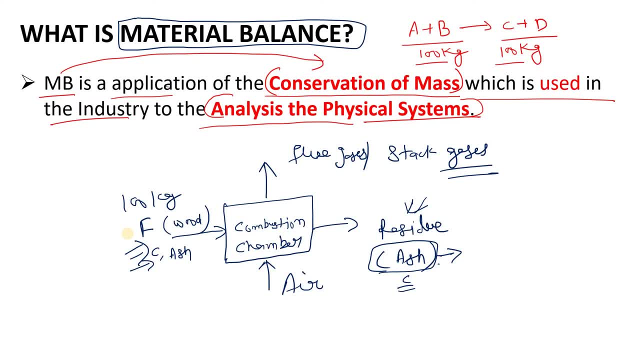 unit operations like distillation, extraction, drying, crystallization, and we will also discuss with the with reaction, like the combustion chamber. okay, so i hope you understood that. what is the beauty of this material balance? we can analyze our physical systems. we can analyze our system. that is our system. we can study that system. you can simply say, with respect to that material inflow: 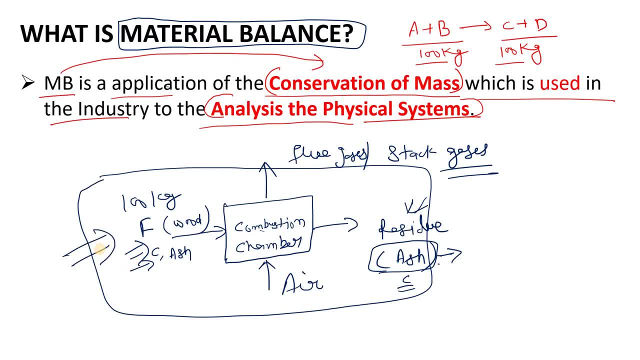 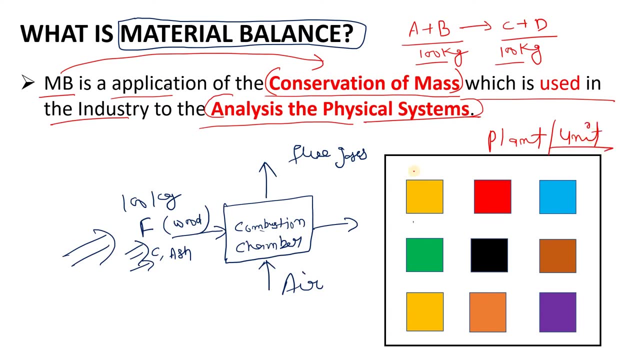 and outflow. okay, this is the first example. what is the second example? okay, here you can see that i just erase this one. okay, let's suppose this is my plant, okay, and i can simply say this: is suppose this is my unit, okay, and this is my equipment number one. 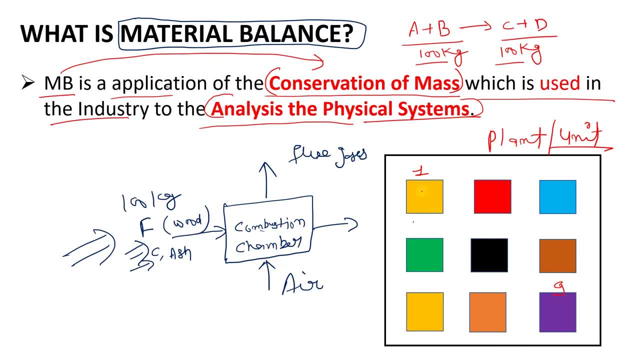 and this is my equipment. number nine means the last, and this is one is beginning and i am supplying some warm material from here and getting the product from here. so with the help of material balance, you can analyze this entire unit. okay, and you can also analyze the individual unit or individual equipment like one, two, three. 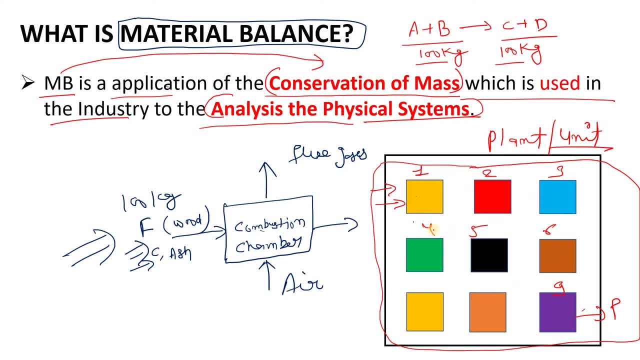 four, five, six so on. got it? my point means you can apply that material balance on the entire unit as well as on the each equipment. that is the beauty. to analyze the our like equipment. or we can say: to analyze equipment means process, okay, like distillation, if suppose. 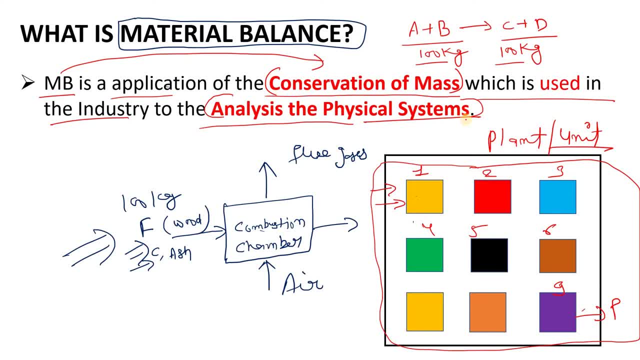 there is a distillation column, so we can apply the material balance on the distillation column. okay, if there is a extraction unit, so we can apply the material balance on the extraction unit. got it? my point means i want to connect you with the industry as well as with the book. i hope you 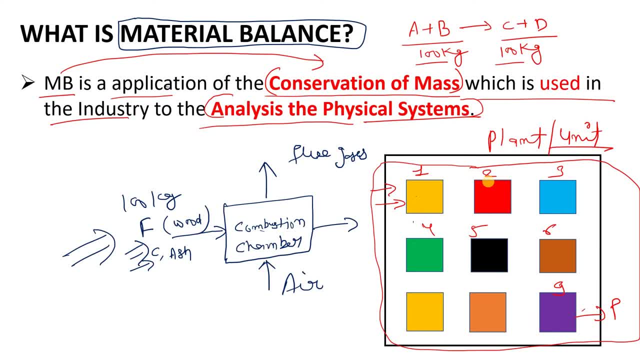 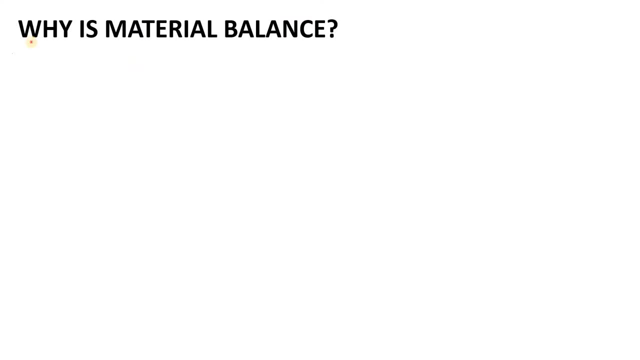 understood that. what is the material balance? and i hope you have now the rough idea what we do with the material balance in the industry, as well as in our like, in our chemical engineering. okay, now let's see. why is material balance okay? why means why we are using this material balance? so, by using the 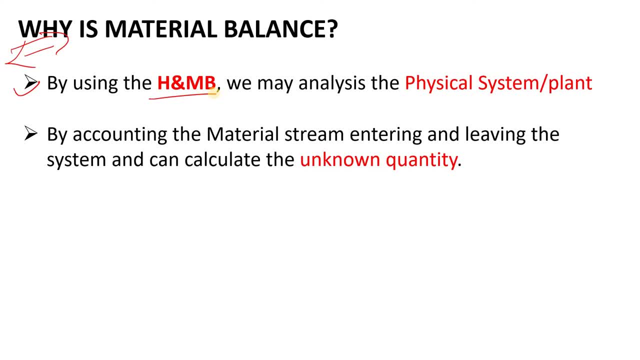 material balance. or you can simply say the heat, and heat and material balance. we may analyze our, like our physical system or unit. okay, like you can analyze the distillation column, okay, you can analyze the extraction unit. you can analyze the dryer. you can analyze the crystallizer: crystallizer. 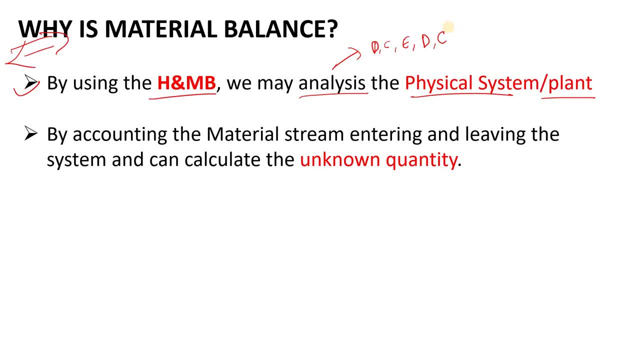 etc. got it my point? analyze means simply you are doing the study, study with respect to material inflow and outflow. second, like you can also count the material stream entering, or you can say the inflow, and the material stream leaving, or you can say the outflow. 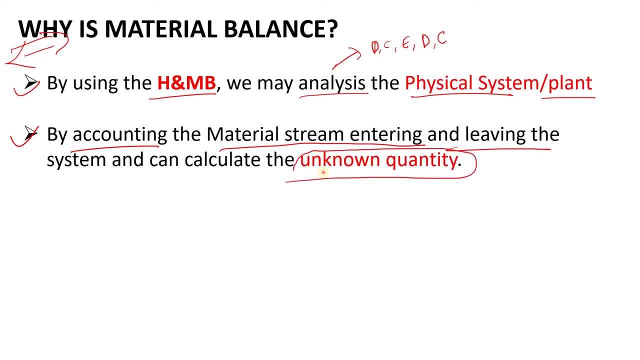 and you can calculate that unknown quantity. okay, suppose here there was the combustion chamber, i was feeding feed f and i was getting residue. okay, in that residue, how much amount of s is there or how much amount of carbon present there? we can find out it with the help of this material balance. okay, 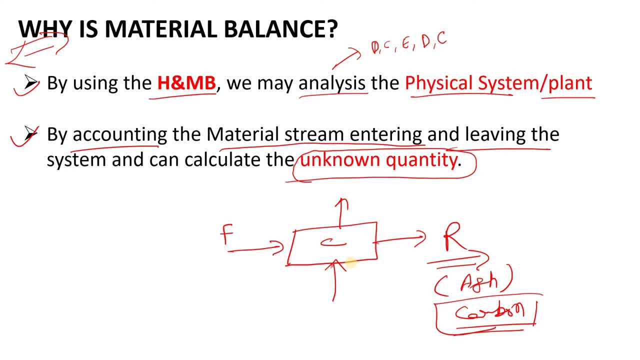 so this is the beauty of the material balance. okay, i hope now you got that why we are using this material balance here. i am using the combustion chamber. you can also analyze here. or you can also take the one example from the distillation column. okay, like in the distillation column, first we feed. 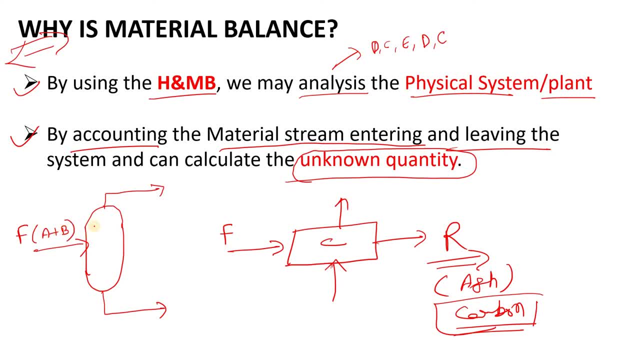 it out and there is a mixture of a plus b, okay, and from here you are getting the overhead product and from the bottom you are getting the residue, or i can say the bottom product. so same we can do with the distillation column. with the help of material balance you can find the unknown quantity. 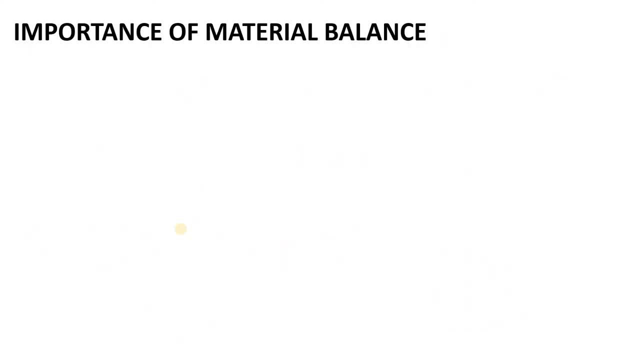 got it now. let's see that. what is the importance of it? if you have understood that two slides, so it will be very, very important, or it will be very easy for you to understand, okay, so the first importance of the material balance is that we may track the 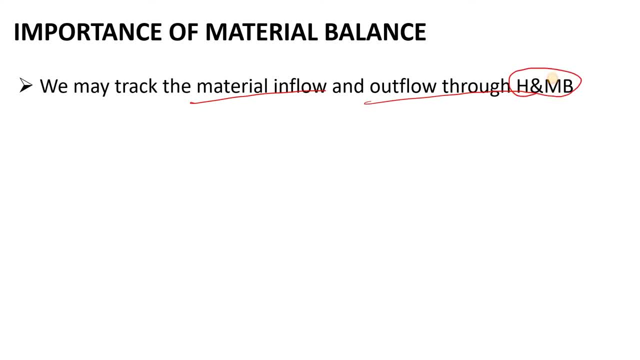 our material inflow and outflow through this heat and material balance. got it my point then. it helps us in the project phases. okay, like suppose if we have to if we are working on the project. okay, if we have to, like suppose here we have to make one unit of the urea plant, okay, so, while making that, 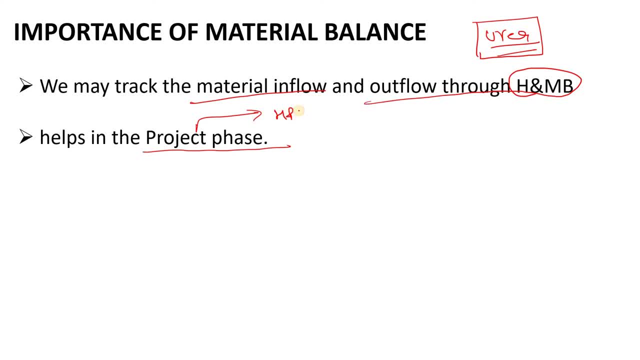 project, this heat and material balance there. heat and material balance help us there to prepare the pn id. okay, like, after the process simulation, we do the like, we make the pfd and then we do the heat and material balance. okay, and after that pfd and heat and material balance, we do the like, we prepare the equipment. process data sheet. 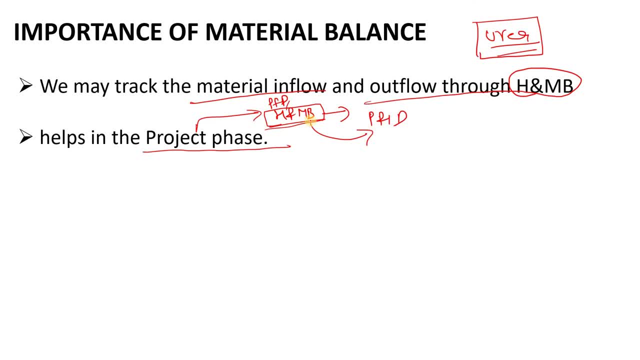 and after that we prepare the pn id so we can say that it helps us in the project phase, got it. and finally, you can simply say that, like, if you are working in our industry, so we can say that it helps us to track the production. okay, like it may be, production of urea, production of ammonia. 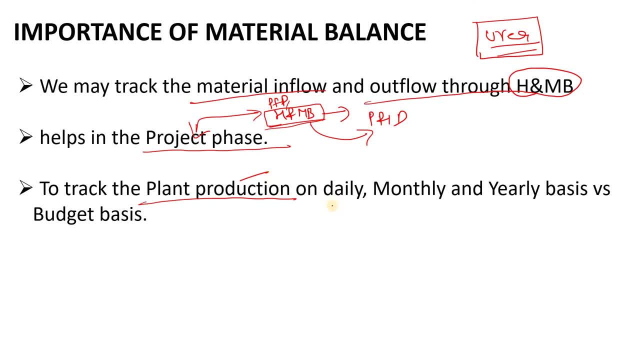 production of naphtha, production of any product whatever, like in which industry you are working. so on the daily basis, monthly basis, you can check. you can check on the early basis as well as versus budget, like what was your budget and how and where you are. okay, you can do that very easily with the 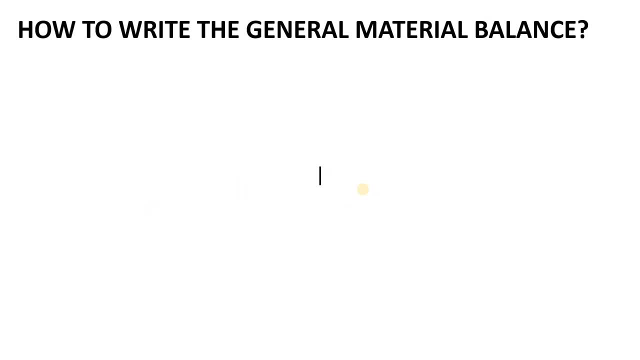 help of material balance. okay, now we will see that- how to write the journal material balance. okay, this is very, very important if you learn it, so you will be easily solved any problem. okay, if there will be some term and condition, you will be easily solved that problem. first, let's go through the 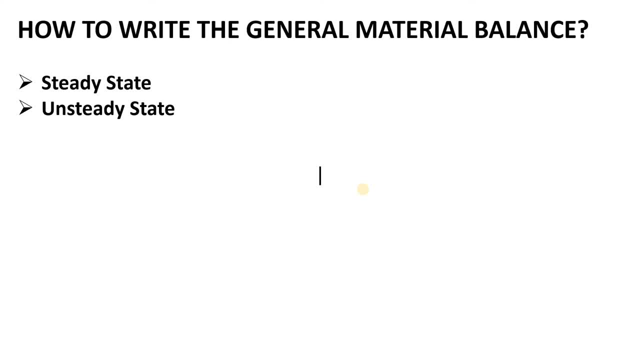 little bit Theory, okay, the first thing is there are two types of material balance. the first one is a study state material balance- okay, where the accumulation term will be zero. and in the unsteady state there is accumulation is not zero. okay, in the case of unsteady state, because in the unsteady 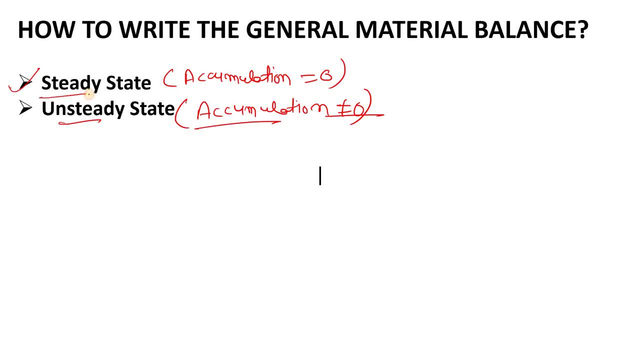 state your variables are going to change with the time, but in study state your variables are not going to change with the time. okay, so first we will discuss or we will go ahead with respect to study state, but in the practice we deal with the unsteady state. okay, so let's go. 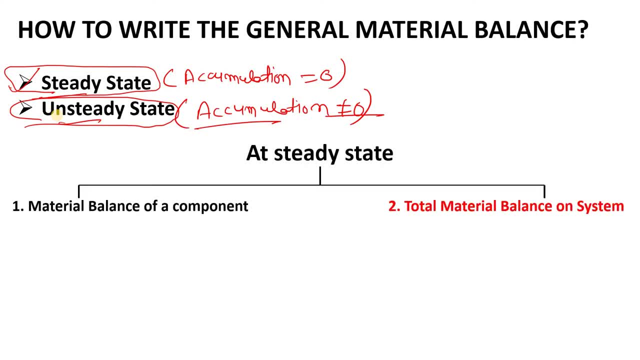 ahead with the study state and at the study state there are two type of material balance. the first material balance we will discuss with respect to material balance of a component means we can apply the material balance on a component, let as we discussed that in our previous example in the 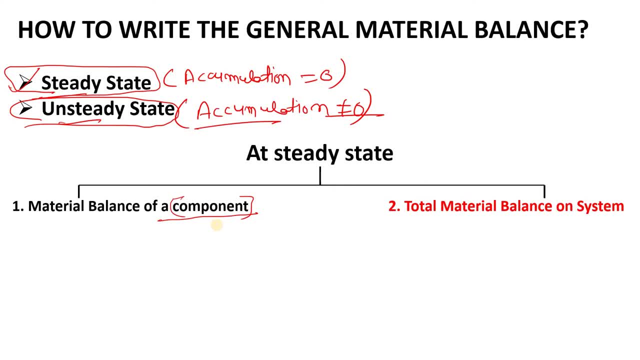 combustion, that we can apply the material balance on the carbon and we can also apply the material balance on the S, okay, and we can also apply the material balance on the on the total system, okay. so that's why here, total material balance on system. suppose it was my. 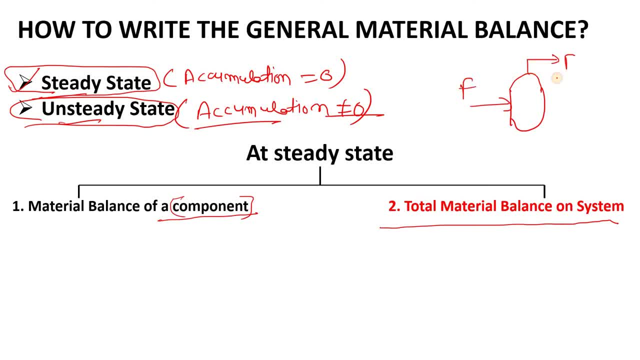 distillation column. so it was F, it was D and it was B. so the total material balance will be: F is equal to D plus B is equal to two points. now it is also further classified and the classification is like that: material balance of a component with reaction, material balance of a component without reaction. 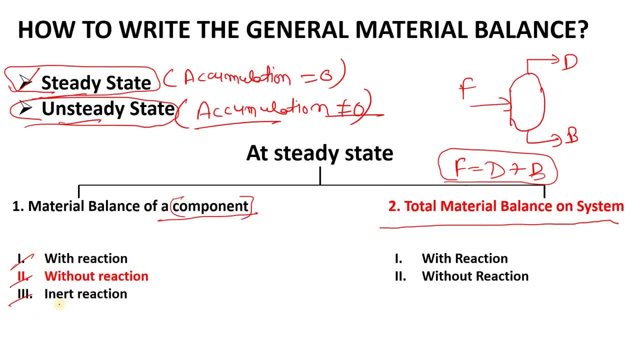 and material balance of component with inert reaction. mainly this inert reaction comes under the without reaction, but we are considering here in a separate subgroup, no problem. and here the total material balance is also classified in two subgroup, that is, total material balance with reaction and total material balance on the system without reaction. 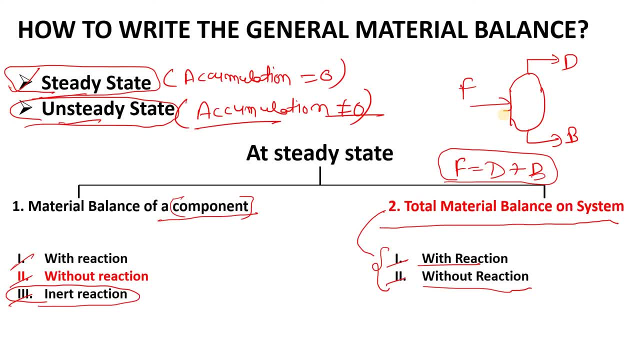 i hope you do not have any doubt. okay, till now. if you have any doubt, you can let me in the comments box. i'll give you the reply as soon as possible and if you are like, if you are enjoying this video, you can also subscribe our youtube channel. okay, so now we will see that. how to write the material. 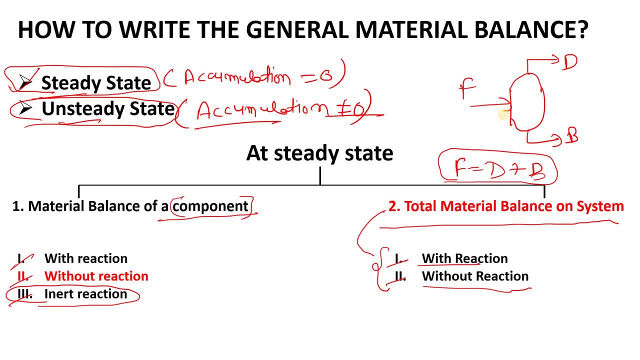 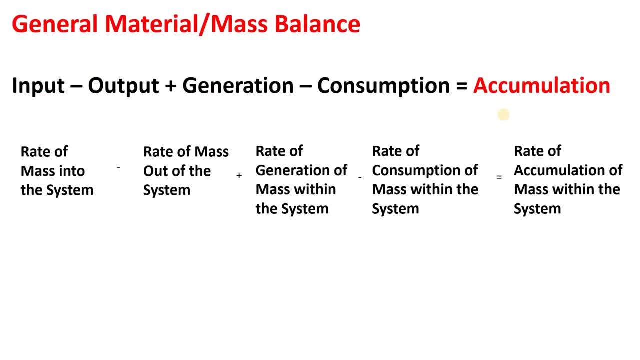 balance. okay, i hope you have understood that. what is the material balance of a component? what is the material balance or what is the total material balance? see here, this is our journal material balance. okay, if you, if you will understand this journal material balance, then you will be easily. 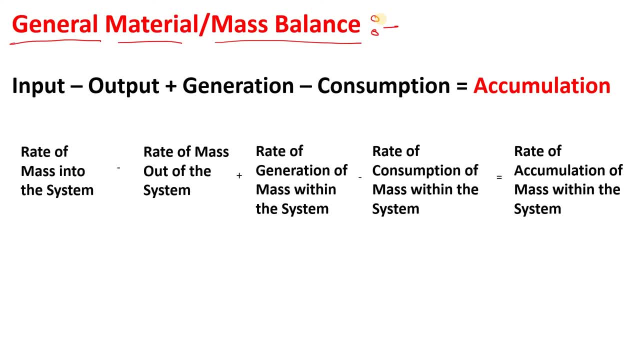 solve any problem. okay, if suppose in the problem there will be some condition, you will be easily solve that problem. there is no, any issue. okay, so the main formula or the journal formula. okay, if there is any, we can say the concept. so for that concept there is one journal concept. 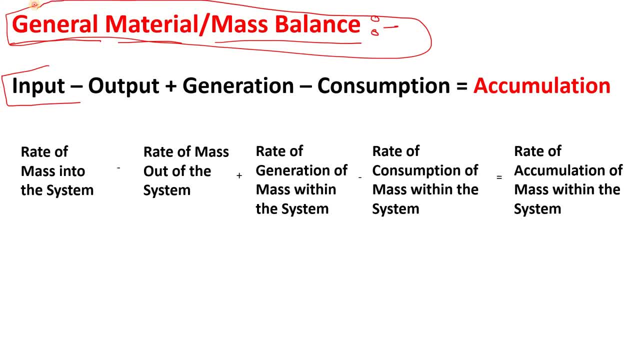 OK, OK, and we can see the journal formula: OK, And after that the conditions apply. So this is our journal formula. OK, And according to that journal formula or the journal material balance, there is an equation: is in minus out, plus generation, minus consumption is equal to accumulation. 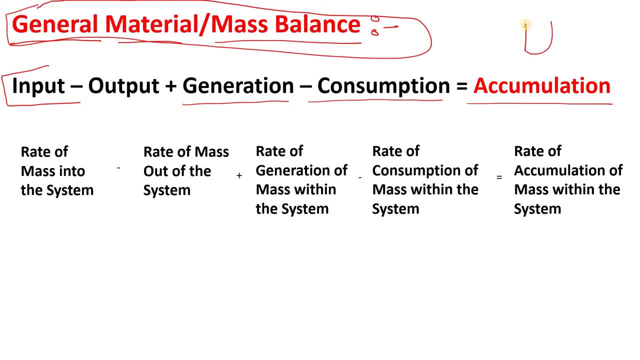 You can relate with this with this distillation column. OK, You can also take any other unit operation, No problem. OK, Now, if we see that, so it will be rate of mass into the system. OK, Rate of mass into the system minus rate of mass out of the out of the system means rate of mass into the system. 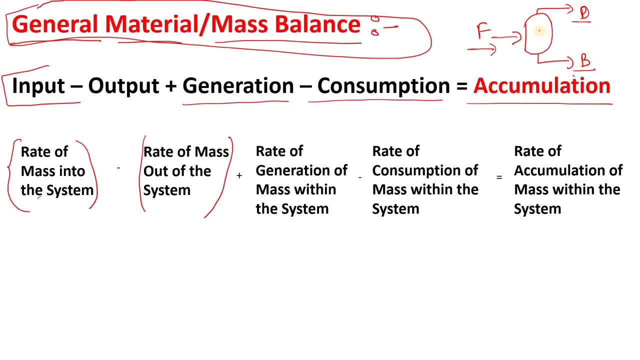 Rate of minus rate of mass out of the system. This is our system, That is, distillation column plus rate of generation of mass within the system, OK. Minus rate of consumption of mass: OK. While in the like unit operation there will not be any reaction. 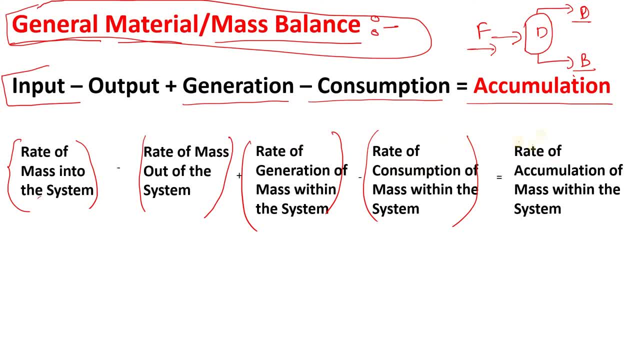 But this is a journal formula. OK, While, like, considering, like, while doing the problem, these terms will be cancelled out or become zero. So that's the another thing. But this is our journal formula, OK, And here is the: and in the last, equal to rate of accumulation. 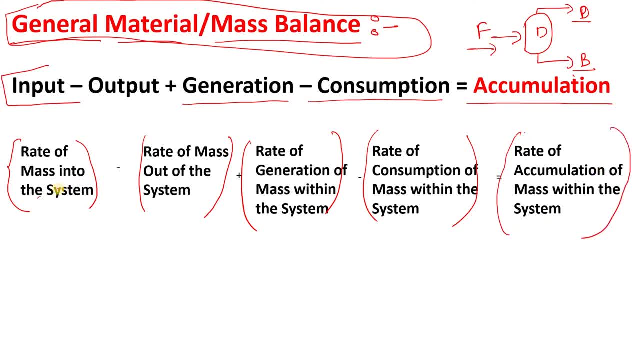 So this is our mass in the system. So this is the number of mass out of the system. So now you understand the second Basically. how is it done? How is the generated mass? Okay, Now we will see how. There is a term called bikers of mass within the system. 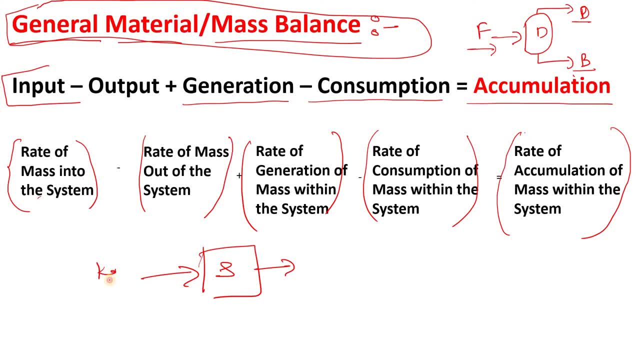 Means? what is the general formula? The general formula is the rate of mass into the system. OK, Rate of mass into the system, The rate of mass out of the system. like rate means KG per hour, OK, KG per hour. 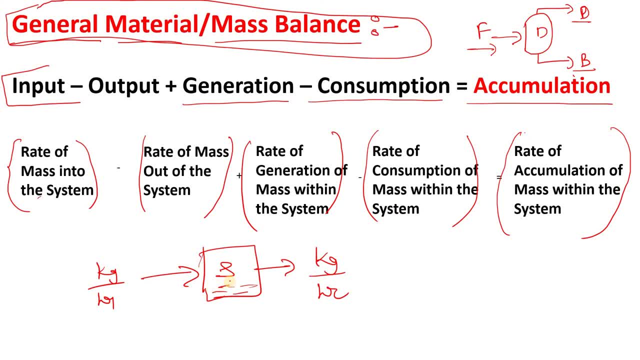 The rate of generation of mass within the system- OK, like how much of how much amount of mass of the system, like mass of the product is going to consume within this system, is equal to rate of accumulation of mass within this system. how much amount of mass is accumulated within this system? this is the journal material balance. now on the 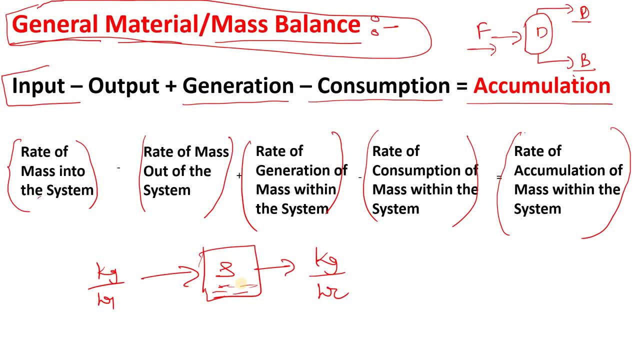 basis of our, like our problem. we can modify or we can arrange this equation. okay, suppose, if you have to, you have to write the material balance on steady state overall mass balance. then this material balance will be changed. what will be changed? this will be zero. this will be zero and 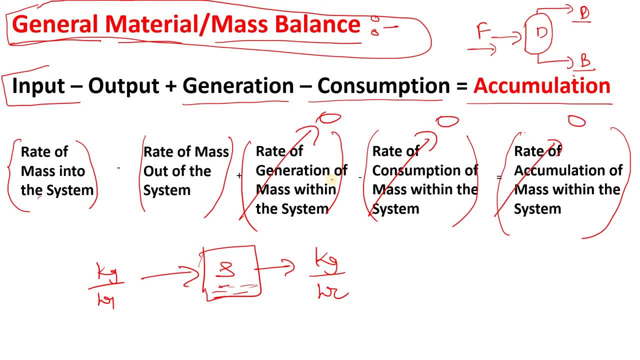 this will be zero. why? because it is a total material balance with respect to steady state, or in the steady state, as i have already told you, accumulation will be zero and in the steady state, the consumption and generation will be also zero. okay, got it my point. same thing that we 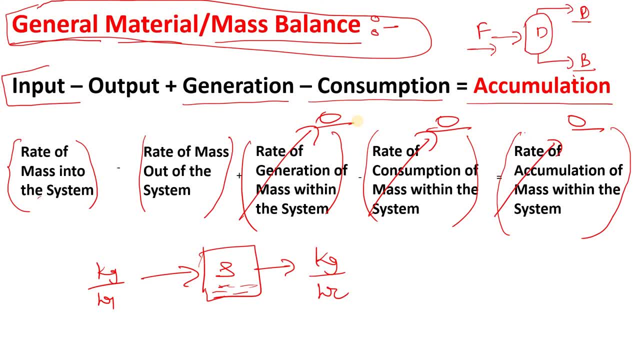 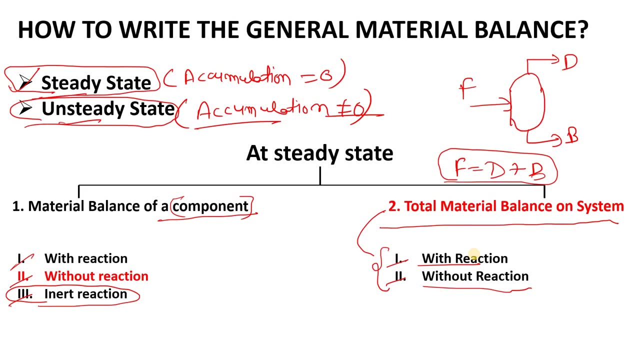 can also apply the material balance on steady state, overall material balance with reaction. okay, then we can also apply the material balance on the innards and we can also apply the material balance on the total system. got it my point, what i want to tell you? okay, so this is the just a. 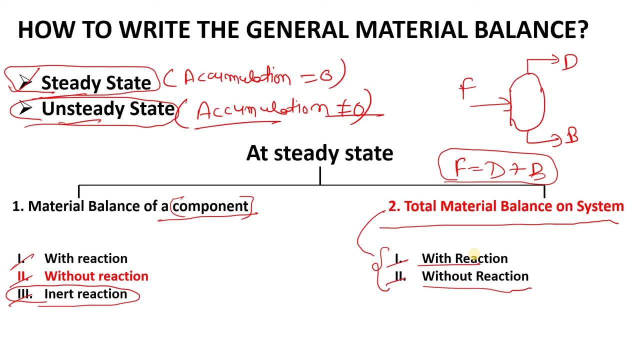 general overview of the material balance. okay, and in our upcoming video, in our next video, we will do the. we will apply the material balance on a specific problem, like steady state over all, material balance with reaction, without reaction, then like steady state over all, material balance with reaction, steady state component, mass balance for a component, which is like taking a part in a 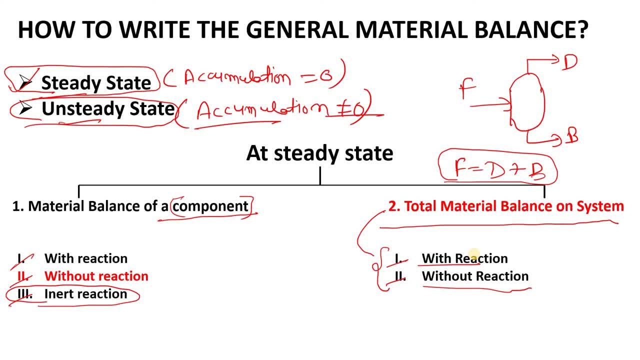 chemical reaction, then steady state component mass balance for a non-reacting substance. okay, in the next video or in our subsequent videos, we are going to discuss about it. okay, you will enjoy this entire playlist. okay, so that was about the material balance. okay, so let's move on to the next. 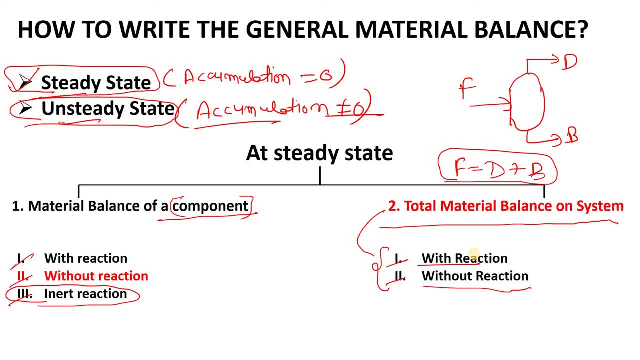 in material balance. if you have any doubt, if you have any doubt in this video, you can let me in the comments box. i'll give you the reply as soon as possible. you can also express your doubts in the comments box if you have any doubts. if you have any doubts in any concept, in process calculation.